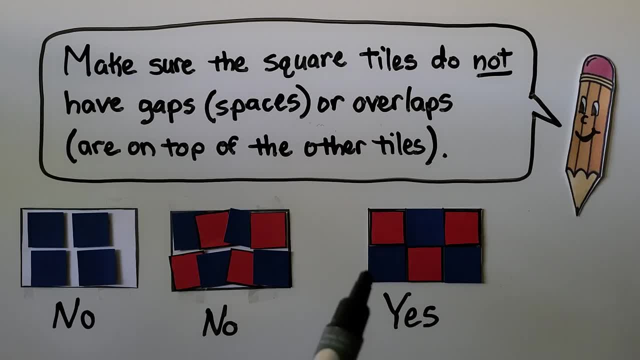 means they're on top of the other tiles, So you want it to be nice and neat like this. We could fit more square tiles here. There's too many big spaces that are left open aren't there, And these are on top of each other. that's too many. 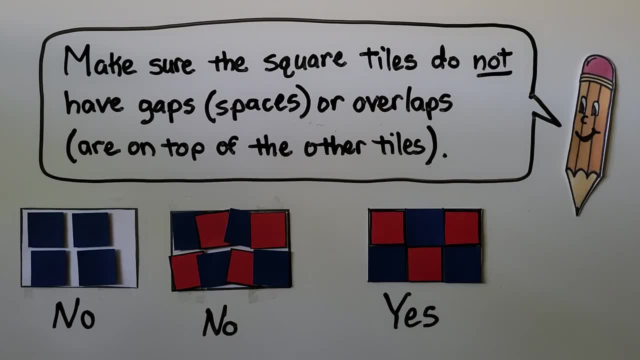 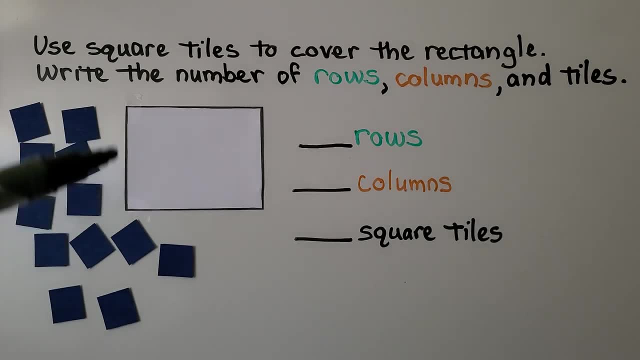 So we want to make sure we do it nice and neat, with no gaps and no overlaps Here. it's telling us to use square tiles To cover the rectangle, then write the number of rows, columns and tiles. We start by putting a tile in the corner up here, then we put another one and we do it. 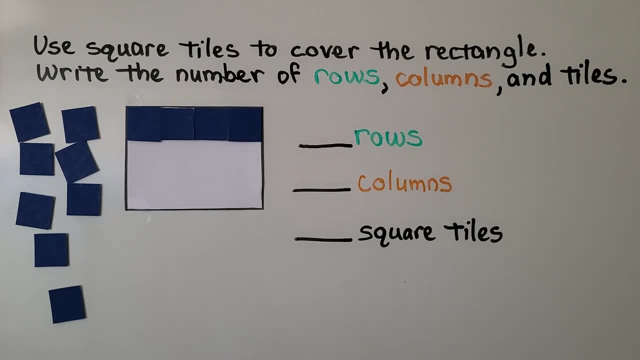 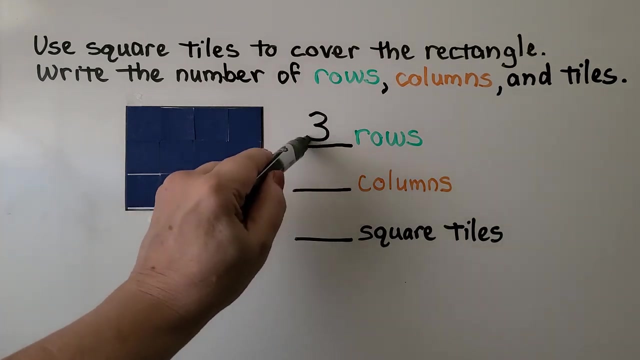 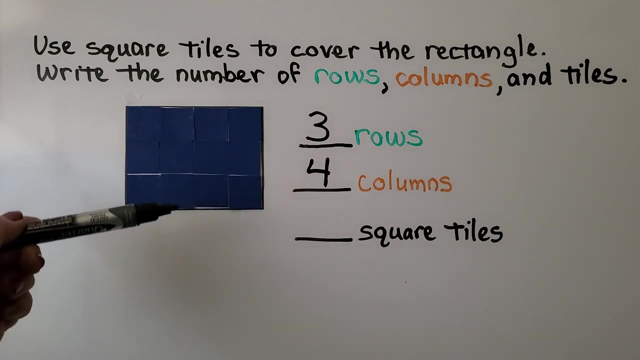 for the whole row. I was able to fit four square tiles in this row. We make another row and I can make another row. I have one, two, three rows. I have one, two, three, four columns. We have four, five, six, seven, eight, nine, ten, eleven, twelve square tiles. 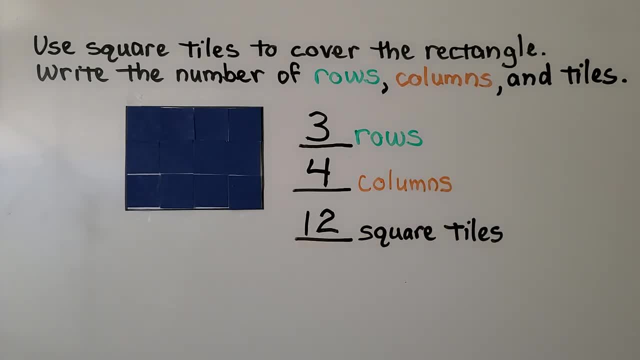 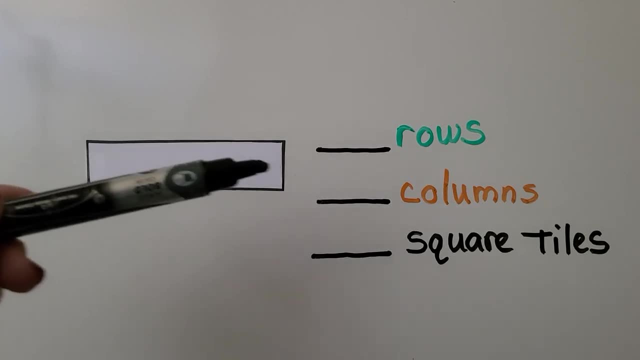 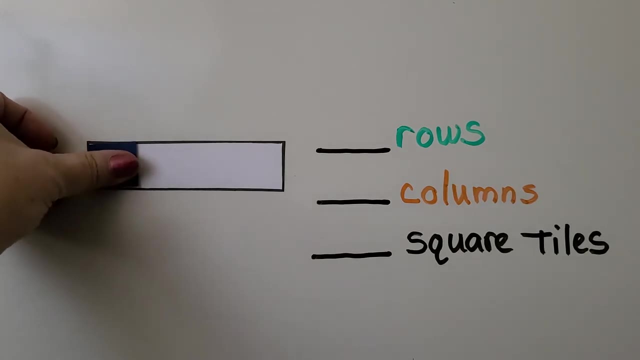 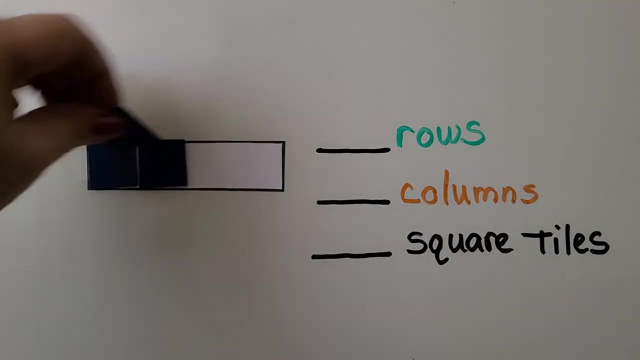 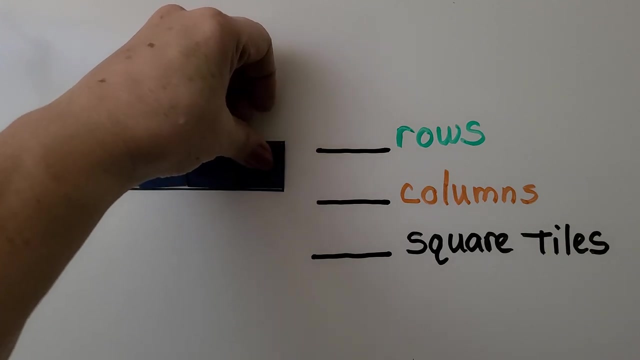 Three rows of four columns. Four columns makes twelve square tiles. This rectangle is very thin, isn't it? It's very long and thin. We start by putting one square tile in this corner and put another one. That's two, that's three, that's four. 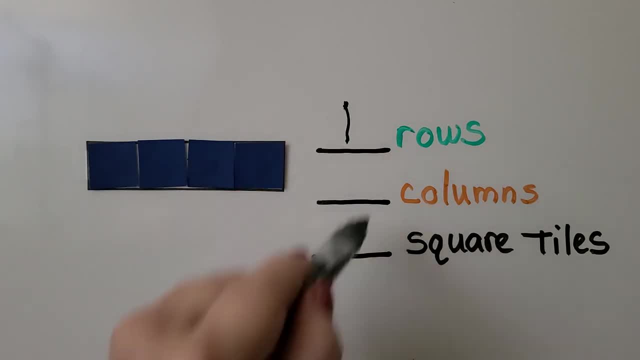 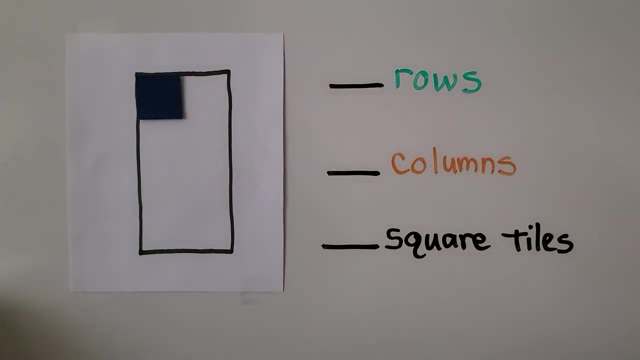 We only have one row, but we have one, two, three, four, five, six, seven, eight, nine, ten, eleven, twelve square tiles. We have four columns. We have four square tiles. Again, we start by putting one in the top corner, like that.